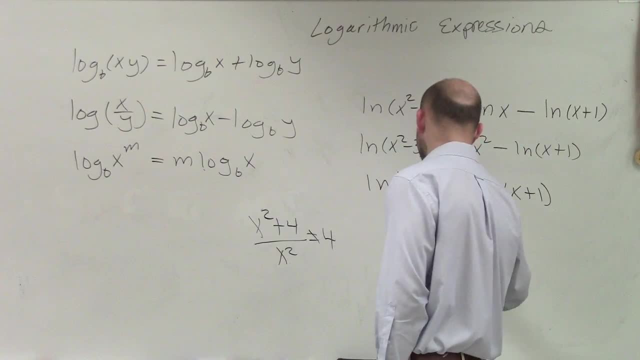 plus 8 divided by 8 does not equal 8.. What's 8 plus 8? 16. 16 divided by 8? 2. 2. 8 plus 8 divided by 8 is equal to 2,, not equal to 8,. okay, So don't just say oh. 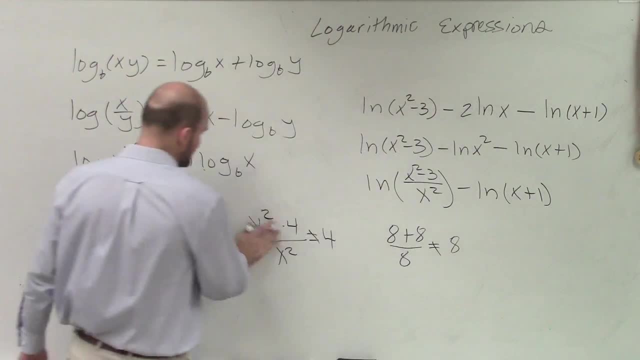 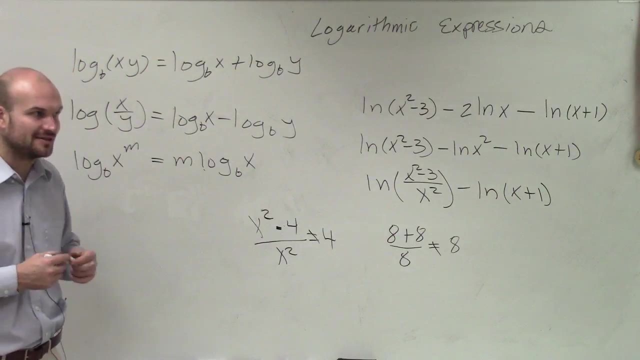 I see 2x squared, so let me cancel them out. Now, if this was like this, where they're multiplied by each other, then, yes, you can divide those to 1.. Mm-hmm, All right, So a big misconception that a lot of students have. 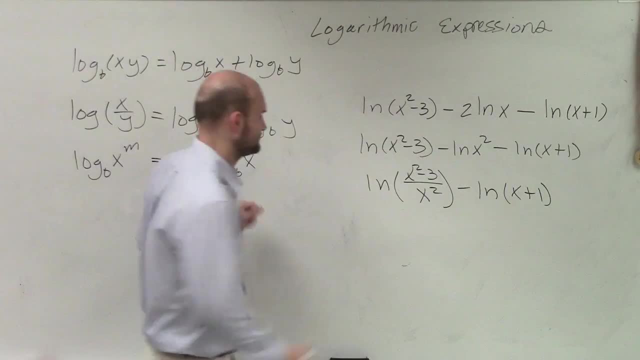 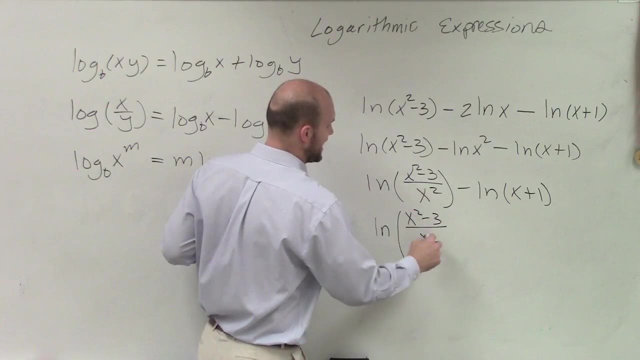 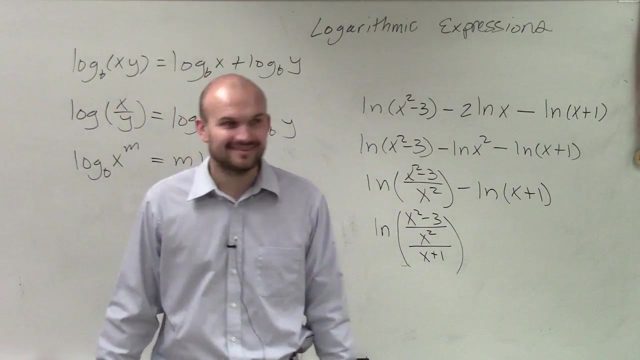 All right, So now we've got to divide this again. Yes, So now it's ln of x squared minus 3, divided by x, squared divided by x plus 1.. Anybody seen a triple fraction? Yes, What class? When? 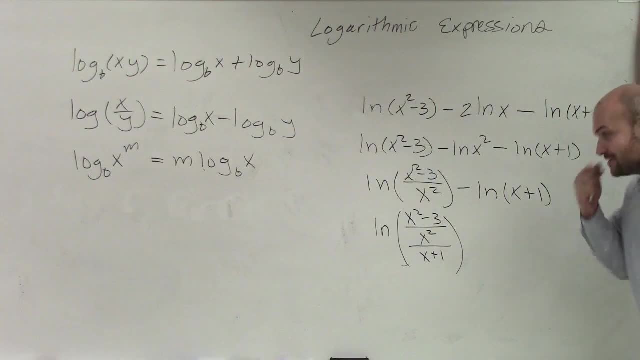 Class 2.. Algebra 2. Yeah, of course You guys should have done these with rational fractions, right, And when we taught these we just went back to fractions, basic fractions. If I have 1 fourth divided by 1 fifth, that looks like this: 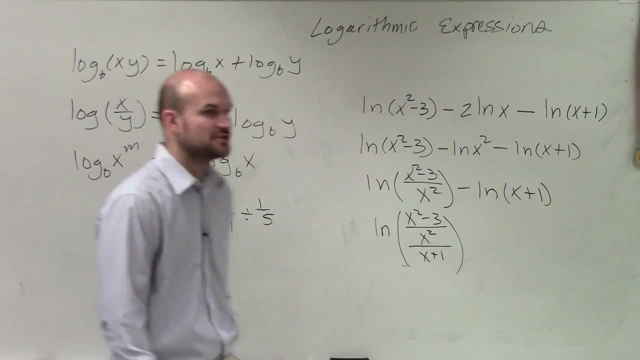 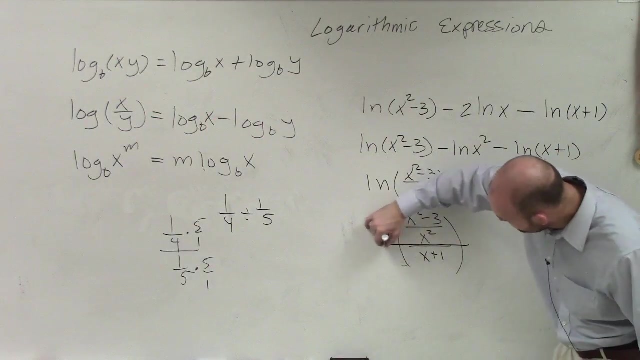 1. fourth, divided by 1. fifth, To get a fraction off the denominator, you have to do what? Multiply by its reciprocal So it gets off. So you multiply by 5 over 1.. All right, So what I like to do is- sometimes I like to extend this- 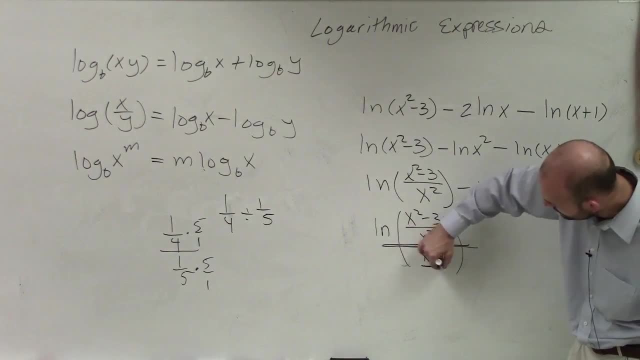 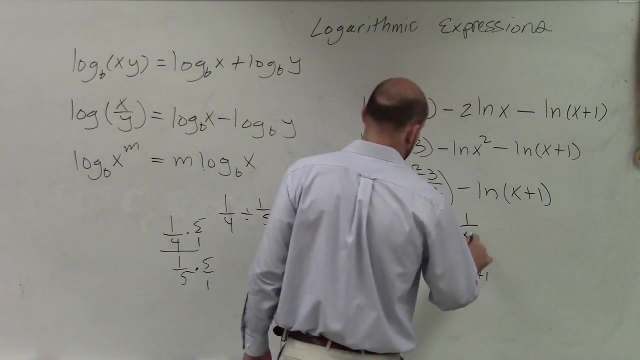 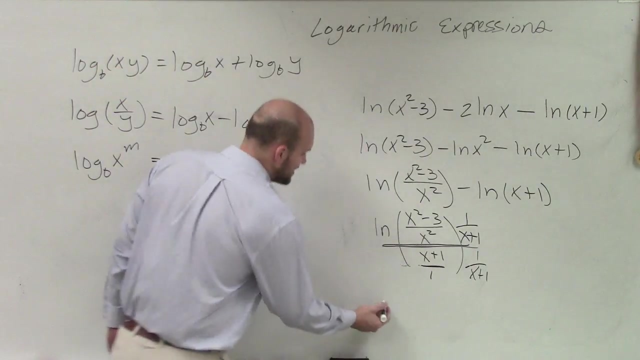 And say it's a fraction divided by another fraction, meaning that's a number that you can put over 1.. Fraction divided by fraction. To get the fraction off the denominator, you multiply by the reciprocal. OK, So now my final answer is ln of x squared minus 3.. 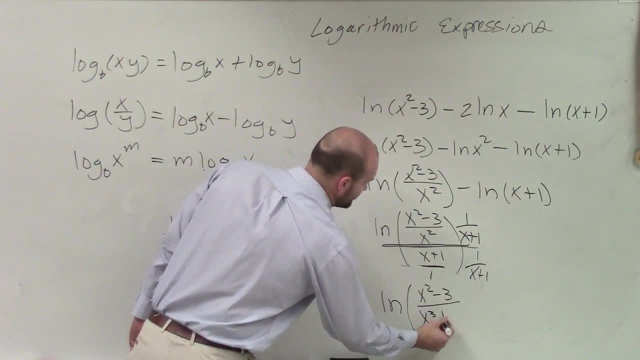 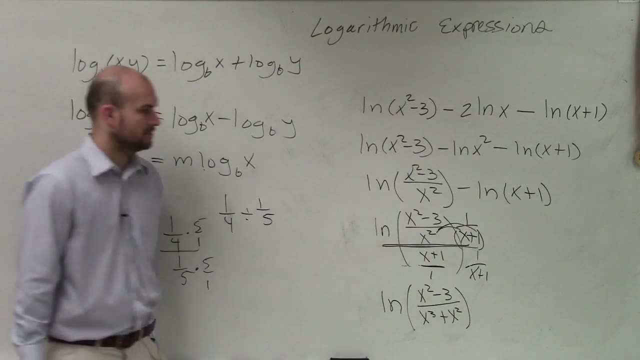 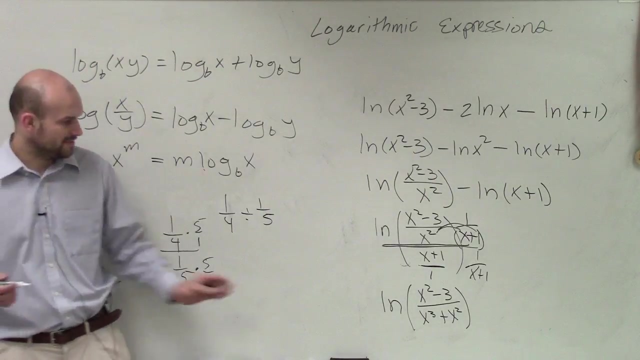 Over x cubed plus x squared as I multiply that out. OK, Cool, Yes, No, Maybe so. So that would be your final answer. Like whoa, Mr McLogan, Whoa, All right, One more.